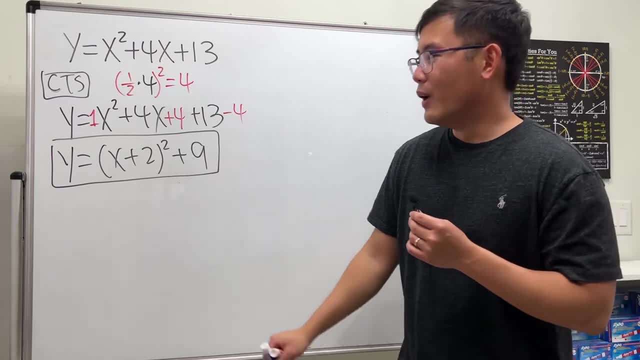 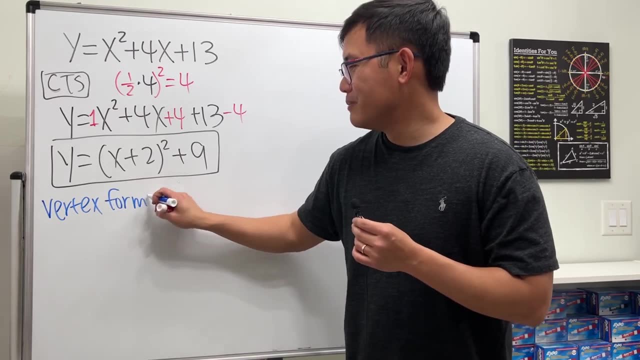 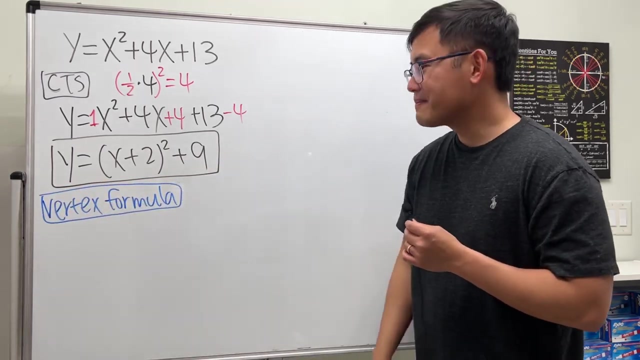 And here's another way to do it. Of course, if you want the vertex form, why don't we use the vertex formula? But I will say this right here is not so legitimate, because completing a square is actually the way to prove that formula right. But anyway. 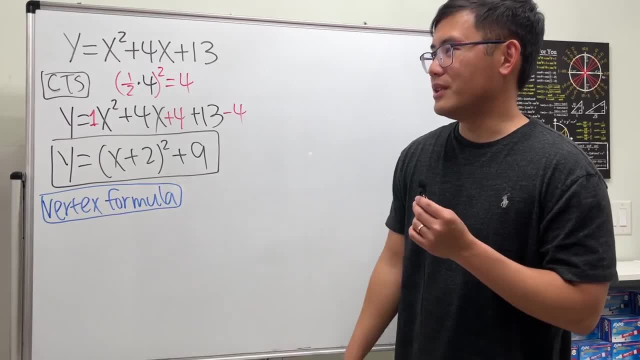 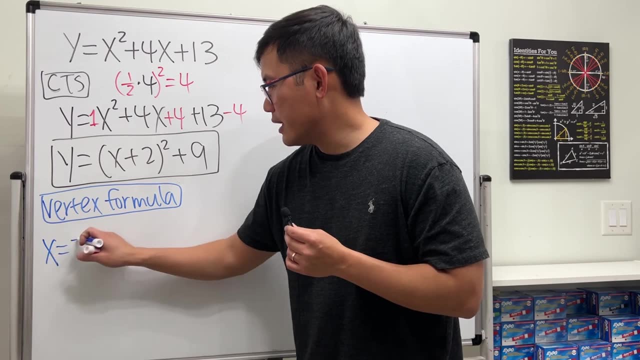 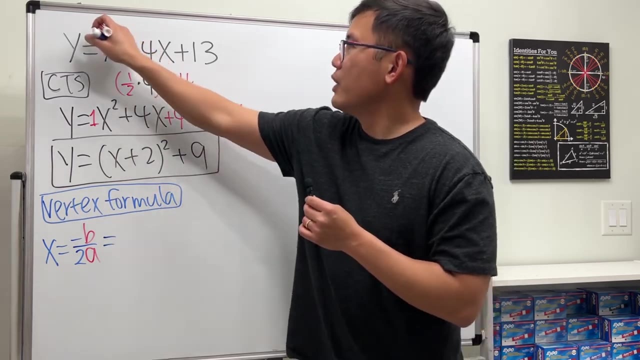 depends on the instruction. If your teacher is okay with using this, then do it. If not, then just complete the square. All right, the vertex formula says the vertex is going to be at: x equals negative b over 2a. right, The vertex formula. Okay, look back here. We know a is equal. 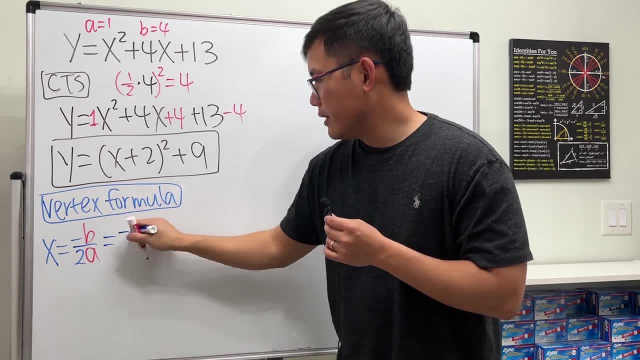 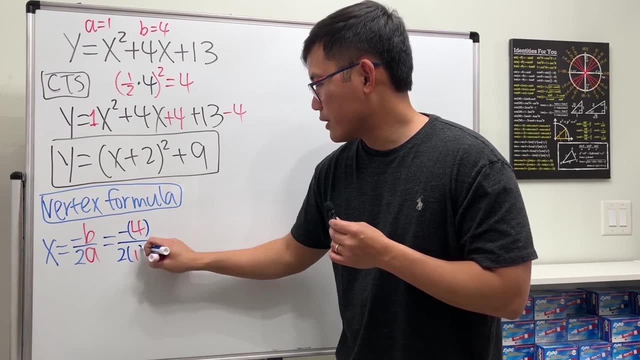 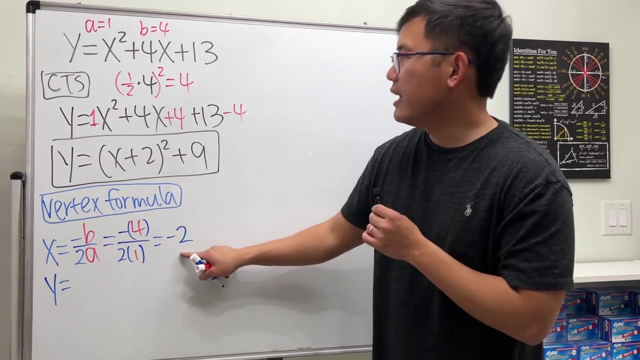 to 1 and b is equal to 4.. So plug in negative 4.. Over 2 times a. Work that out. we get negative 2.. This is just the x. We also need a y. Y is going to be plugging negative 2 into the original and then just plug into the x. We have negative 2. 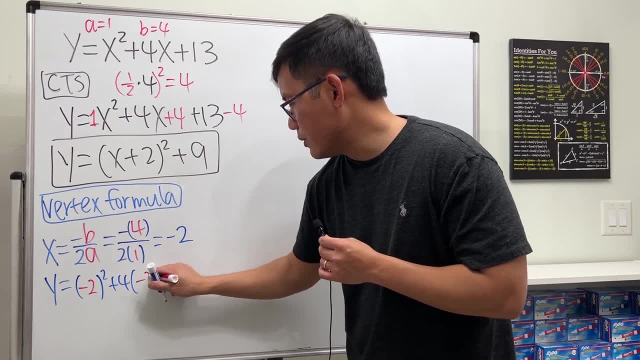 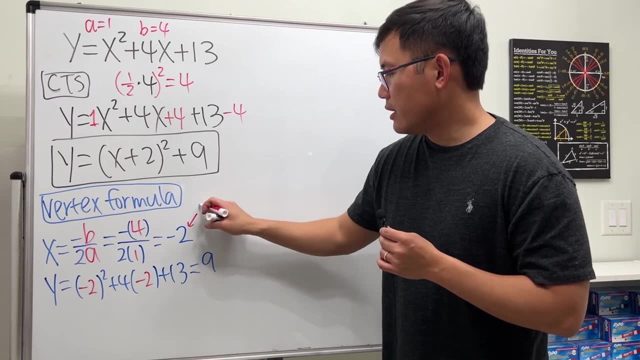 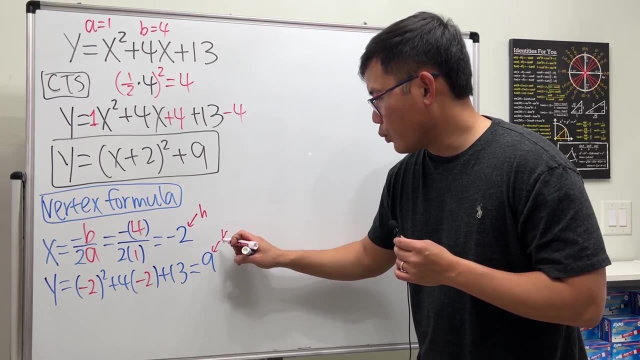 squared plus 4 times negative 2, and then plus 13.. Work that out, we get 9.. This right here, it's the h value, which is the x coordinate of the vertex, And this right here is the k value, the y value of the vertex. 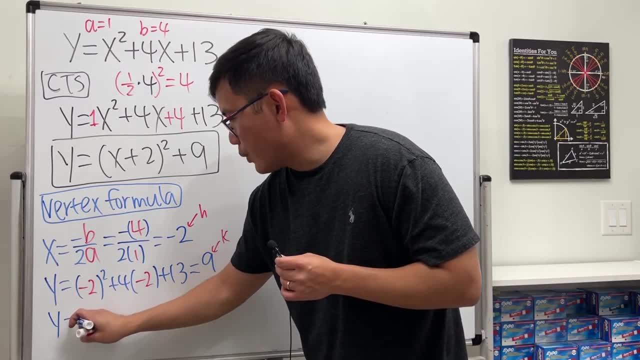 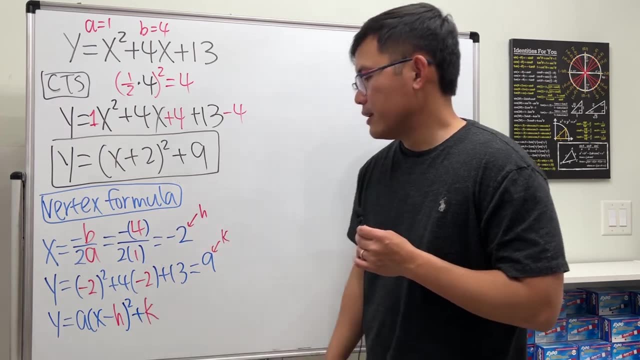 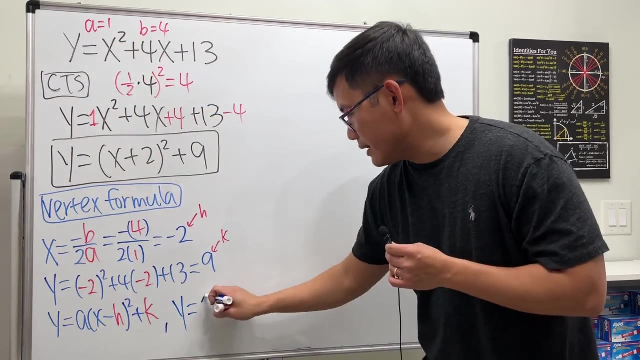 And the formula is: y is equal to a times x minus h squared plus k. So of course we can just put everything in now. So we have: y equals a is still the same as that, So it's just 1 times x minus. 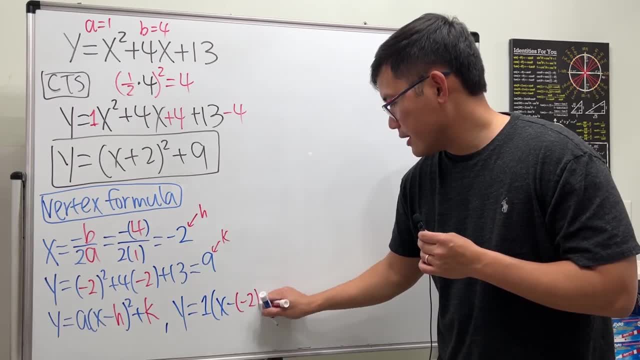 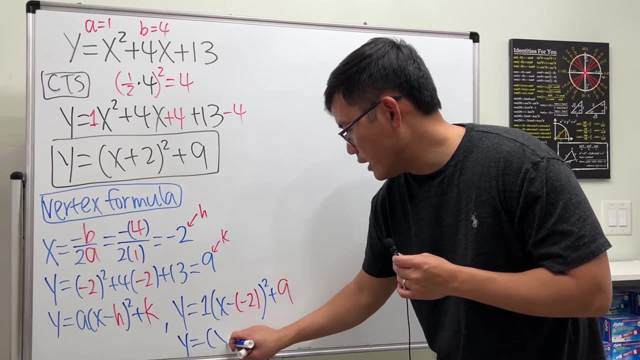 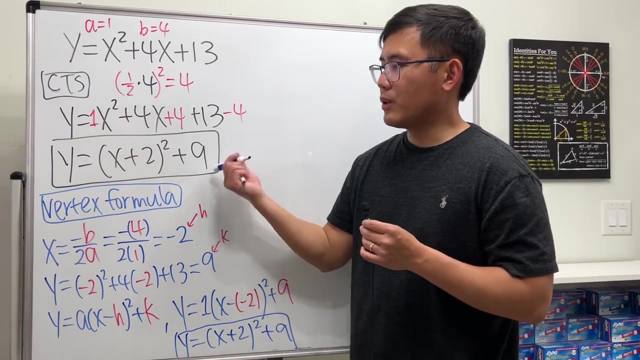 negative 2.. Square plus k, which is 9.. And of course the 1 doesn't matter. You can just write: y equals x, and then plus 2 squared, and then plus 9.. And here is the vertex form, just like what we got. 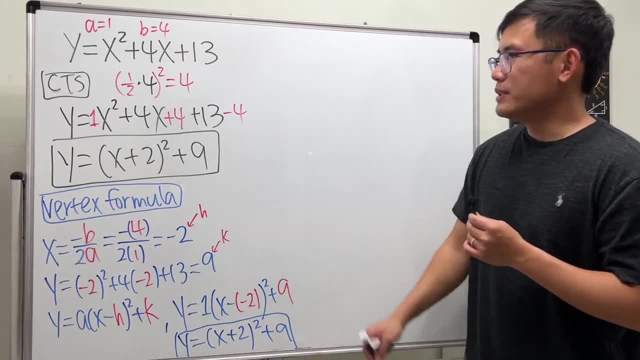 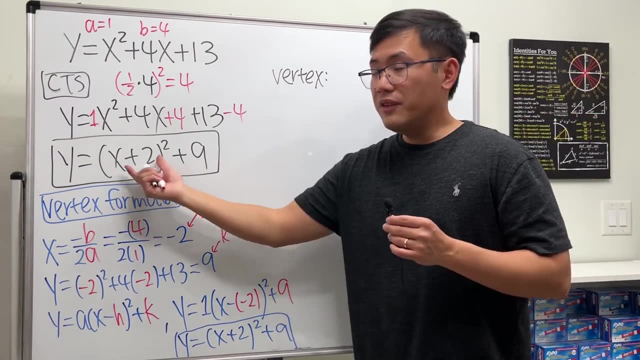 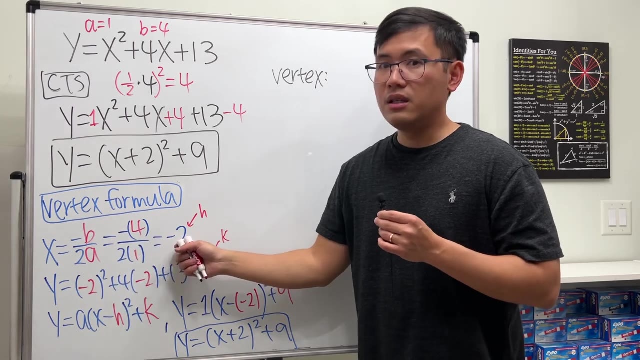 earlier, Same thing, of course. Now let's make a quick sketch. We know the vertex is what? Negative 2 comma 9.. If this is what you have, make sure that you do the opposite: negative 2.. Otherwise, worked out the formula, you can see that it is indeed negative 2.. How can you make this?